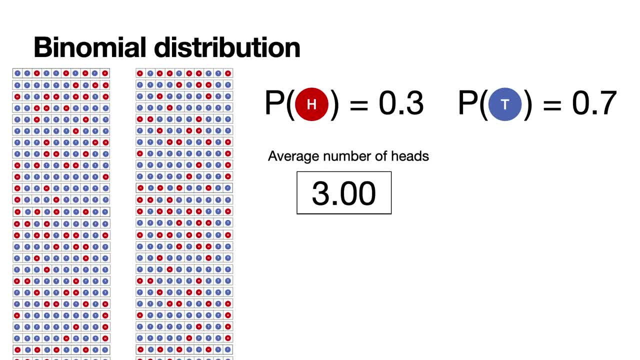 let's run it hundreds and hundreds of thousands of times. and what happens? well, when we run it for a long time, with lots and lots of tries, we can see that the number converges to three heads, which makes sense. this is the limit. so now we get is this: 3, which is 0.3 times 10, which is the probability of landing in. 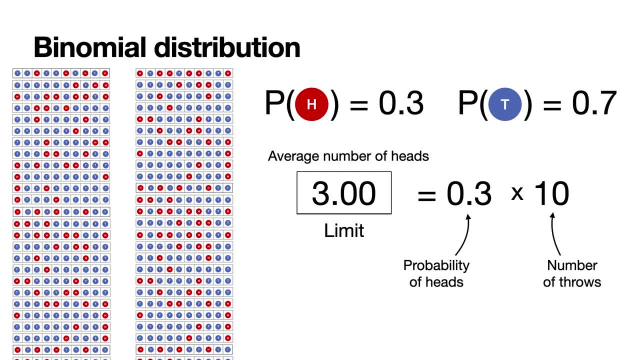 heads times the number of throws in each run, and this is what happens in general. the probability of the coin lands in heads is P, and in each run we throw the coin n times, then the average is n times P, and this is what we call the expected number of heads. so now let's look at the probability of getting. 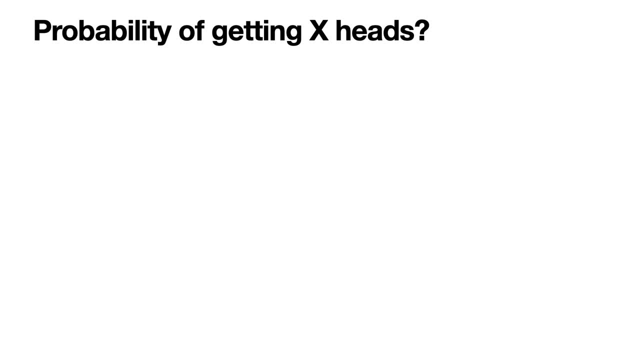 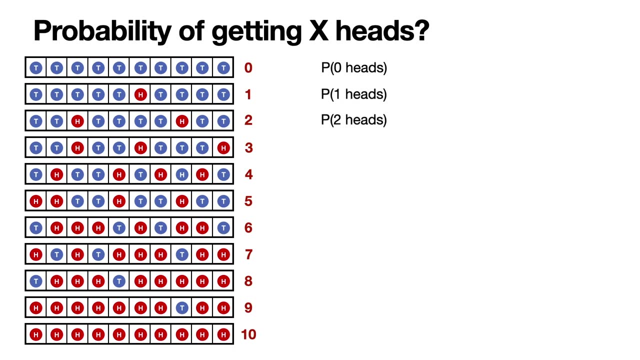 any number of heads and we throw the coin 10 times. if we throw the coin 10 times and 11 things can happen, because the number of heads can be 0, 1, 2 or all the way until 10, and for each one we're going to calculate the probability. 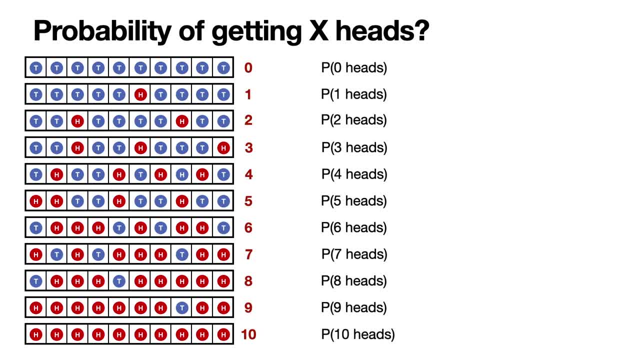 and I'm going to first give you the numbers and then show you how to find them. the numbers are these ones over here, and you can verify that they add to one, because these are all the possible cases. now, for each of the cases, we've highlighted one particular possibility, but think of all the ways a coin could. 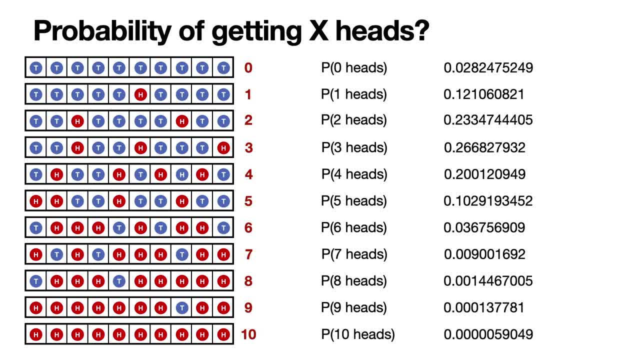 land in each particular number of heads. for example, in the first case where it was one times heads. this can be in the first throw, or it can be in the second throw, or in the third one, or in any of the throws. now also notice that the highest of these probabilities is for three heads. 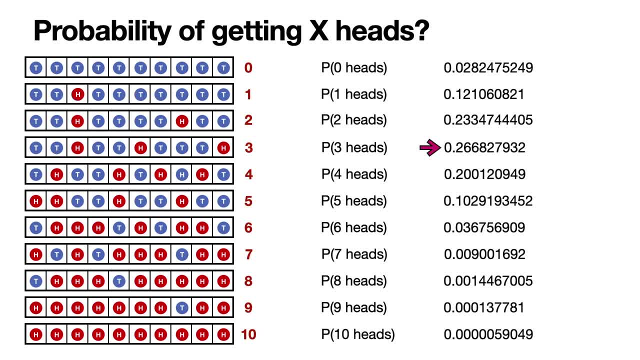 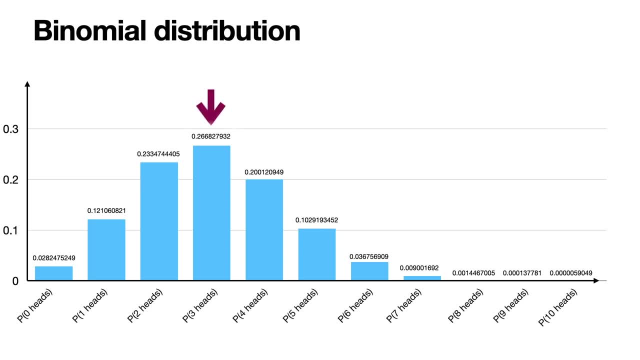 and that makes sense, because the probability of landing in heads is 30. so what I'm going to tell you next is how to calculate all these 11 numbers, but before calculating them, let's put them in a plot like this. notice, this time is visually, that the event with the highest probability is that the coin. 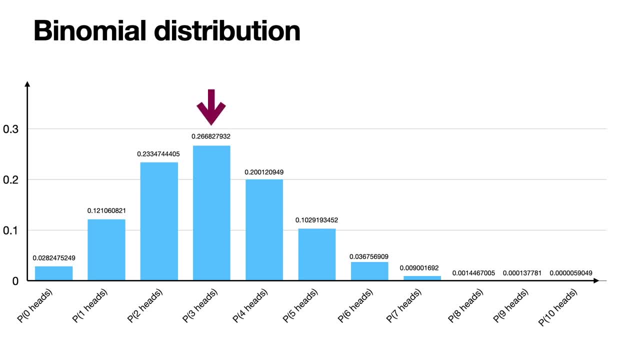 lands on heads three times out of ten. in this histogram you can see that on the horizontal axis you have zero heads, one heads, two heads, all the way to ten heads, and on the vertical axis you have the probability. so this is plot is precisely the binomial distribution. the parameters of this binomial distribution are the. 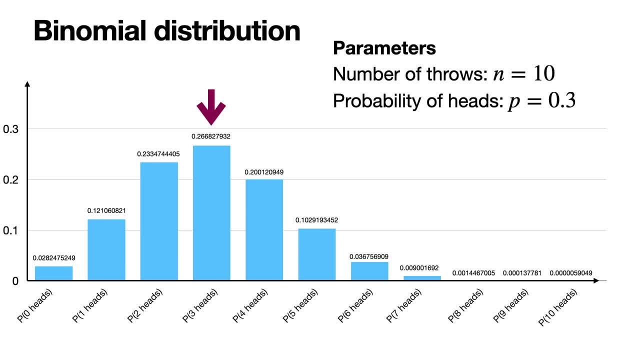 number of throws, n, which this this time is 10, and the probability that a coin lands in heads, which this time is 0.3. if we were to change the parameters of the distribution, the histogram will change, but it's always going to look like something like this, with a bump in the middle, in fact, as n tends towards. 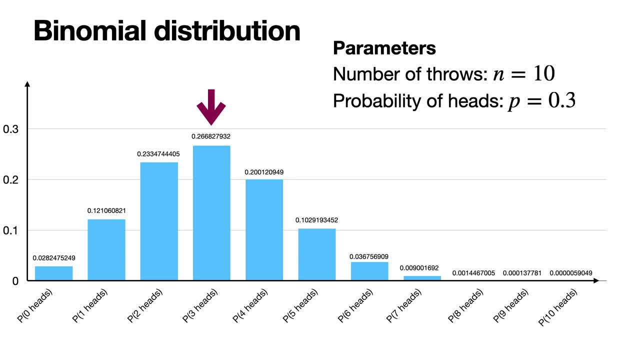 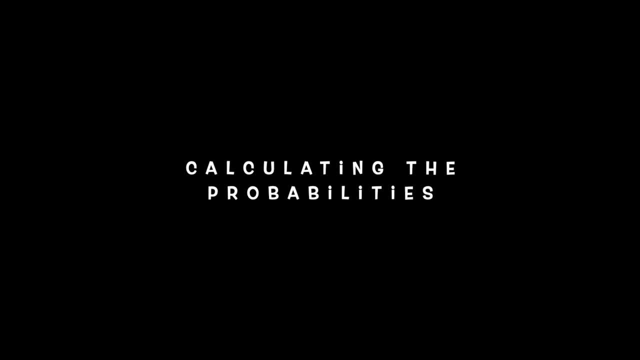 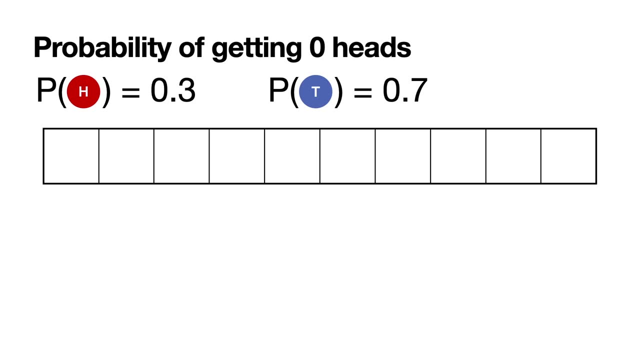 infinity. the binomial distribution tends to a normal or Gaussian distribution, something called the central limit theorem, but that will be a topic for another video. okay, so, as I promised, I'm going to show you how to calculate these probabilities. so here it goes. first let's calculate the easiest one, which is when the coin lands in head. zero times, that means. 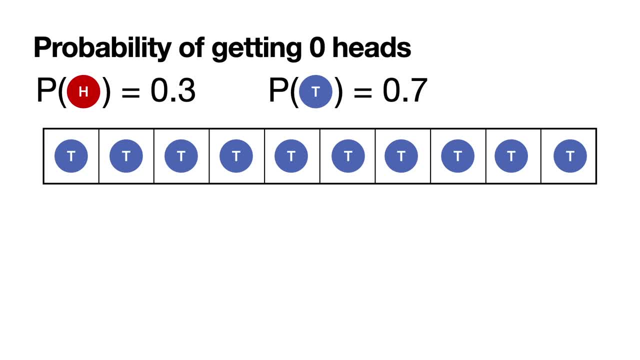 each throw must land in tails, and the probability of the coin landing in tails is 0.7 for each of the throws. since the throws are completely dependent from each other, then we multiply this probability to obtain the total probability. so the answer is 0.7 to the power of 10, which is 0.02825. 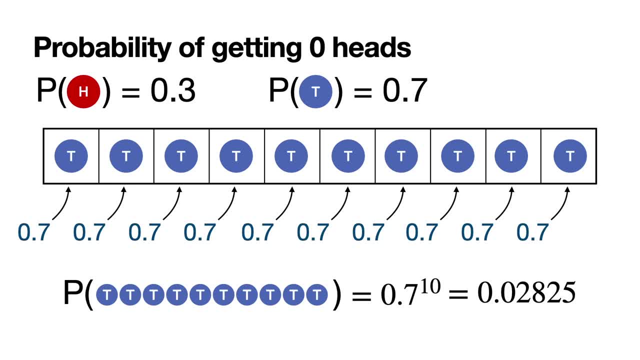 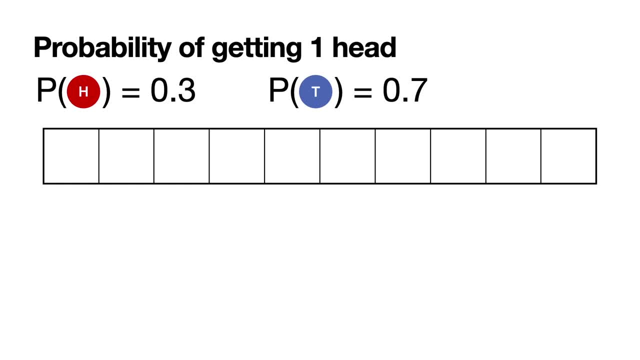 this is quite small, but that's the probability that all of them land in tails, so that we have zero landing in heads. now let's do one a little bit harder: what's the probability that only one of the throws lands in heads? before answering that question, let's answer a simple one: what? 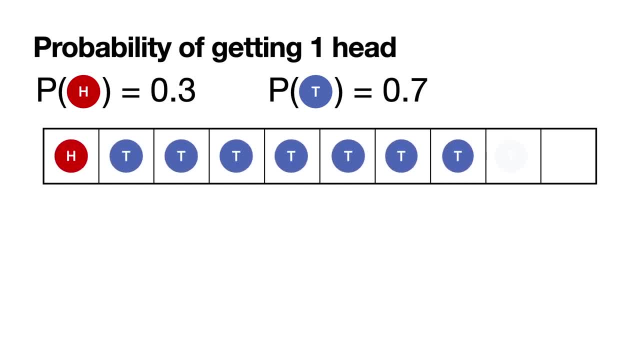 is the probability that the first throw lands in heads and all the other ones land in tails. well, for the first one to land in heads, the probability is 0.3 and for the remaining nine that land in tails, each one has a probability of 0.7. therefore, the probability of those all 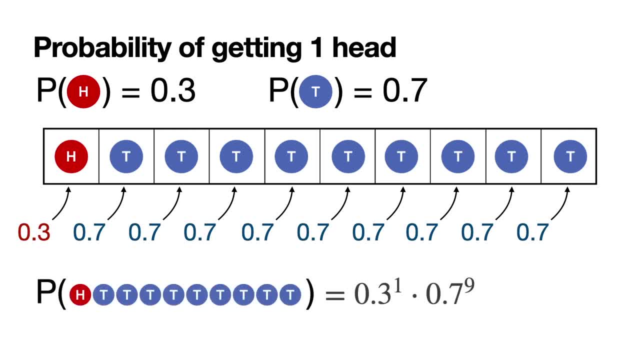 these events happen in that order, since they're independent again, is 0.3 to the one that's for the heads times, 0.7 to the power of nine for the nine tails, and that number is 0.012106. now, remember that this is not all. this is the probability that the first throw 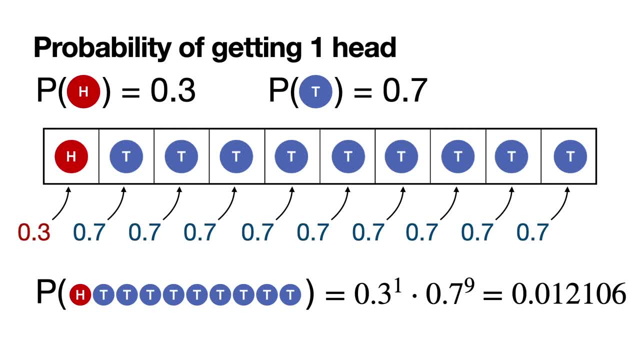 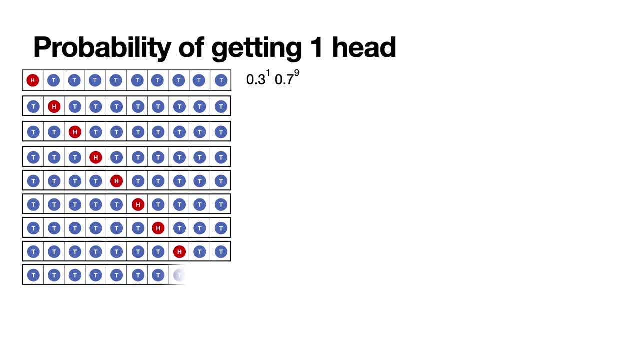 lands in heads. we're still missing the probability that any of the other throws is the one that lands in heads. so let's look at those. there are 10 ways in which one of the throws can land in heads and all the other ones in tails. and here they are. the throw that can land in heads is can be the first. 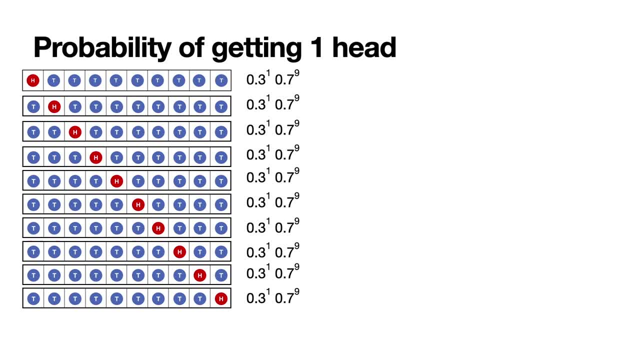 one, the second one, Etc, Etc, until the last one, and all of them have the same probability, because all of them are: 0.3 to the one for the heads times, 0.7 to the nine for the nine tails. now, since these events are disjoint, namely no two of them can happen at the same time, the 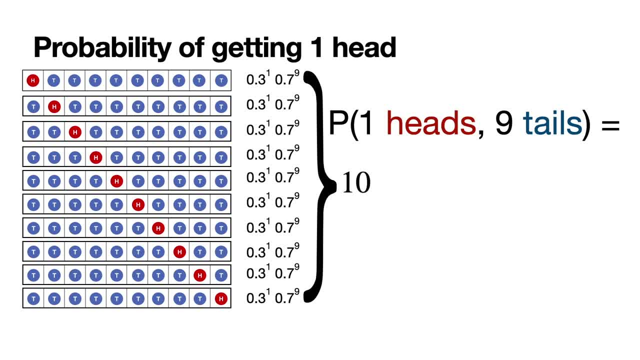 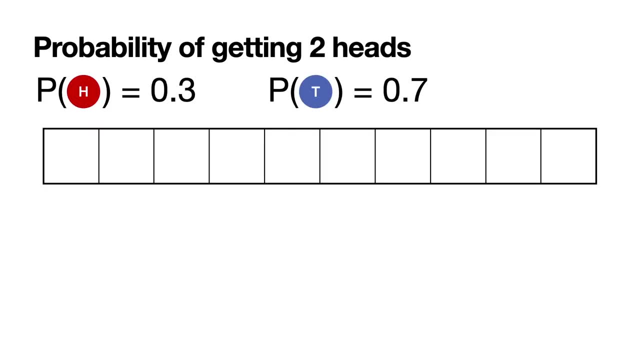 properties now get added, and there are 10 of them. so therefore, the probability that one coin lands in heads while all the other ones land in tails is exactly 10 times 0.3 to the one, times 0.7 to the nine, which is 0.12106. and now let's do the same thing for two heads. so let's start by considering: 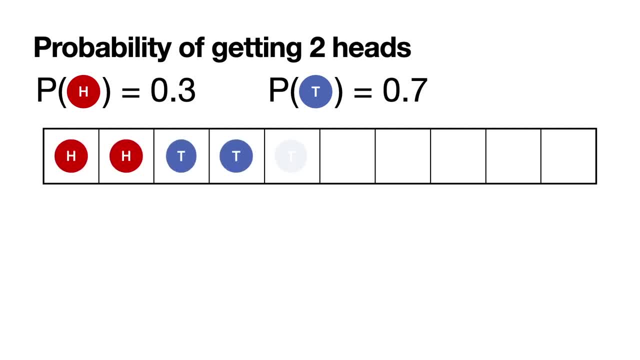 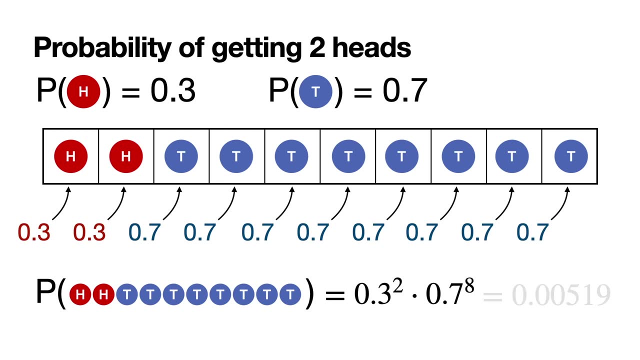 the probability that the first two throws land in heads and all the other ones land in heads. that probability calculate in the same way as before. it's going to be 0.3 squares times 0.7 to the eight, and that's for the two heads and the eight tails, and so this number is 0.00519 now 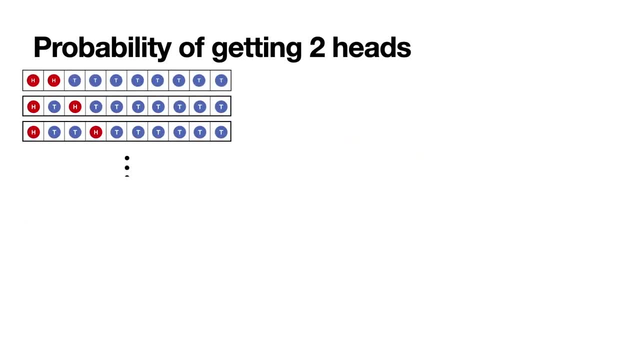 the question is: in how many different ways can we have two heads amongst 10 throws? the number is 45. why 45? because 45 is the number of ways of picking two objects out of 10, also called 10: choose two. all of these have the same probability as we saw before, so the probability of two heads. 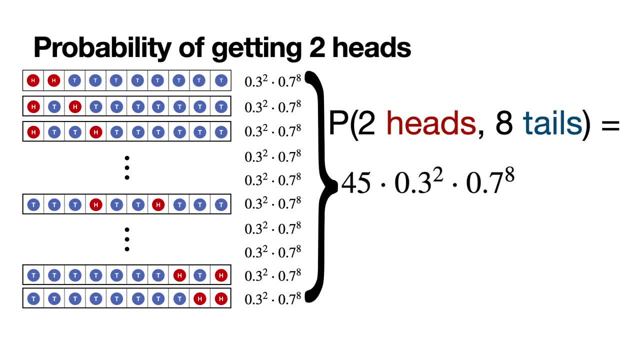 eight tails is going to be 45 times 0.3 squared times 0.7 to the eight, which is 0.12106, as I mentioned before, this 45 is 10. choose two the number of ways to pick two objects from a set. 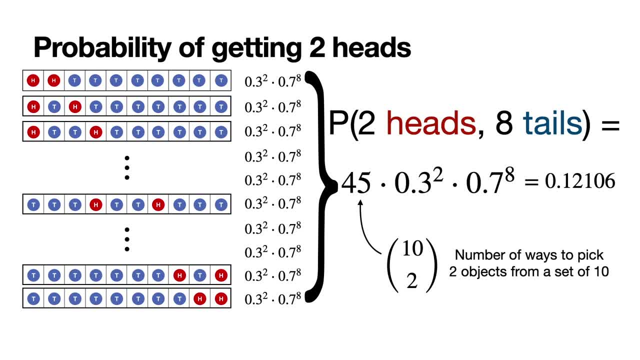 of 10, and those two objects are the two positions in which the coin lands in heads and that also determines the eight that land in tails. this number happens to be 10 times 9 divided by 2.. why? well, because we have 10 possibilities for 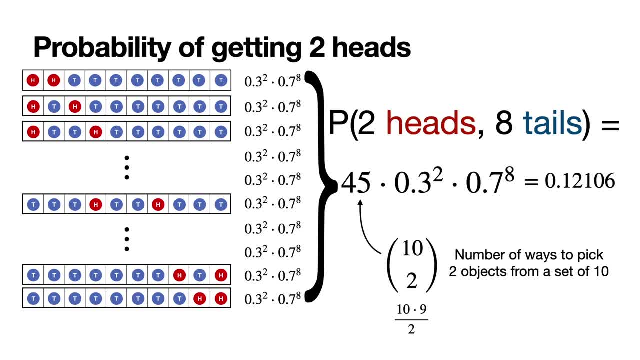 the first position of the ages of the heads and nine for the second one. so one is taken already. and also we are counting them all in two different ways, because we're first counting the first coin on the second coin, but we're also counting it as the second coin and the first coin. so we're 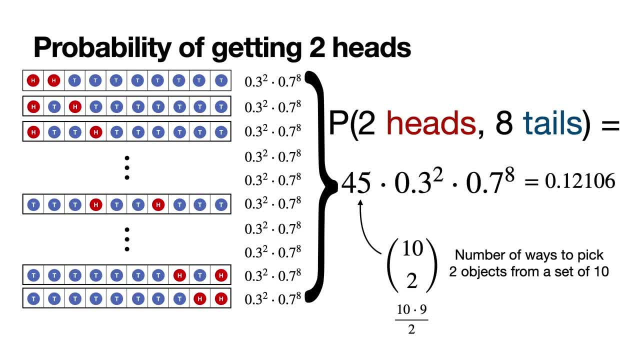 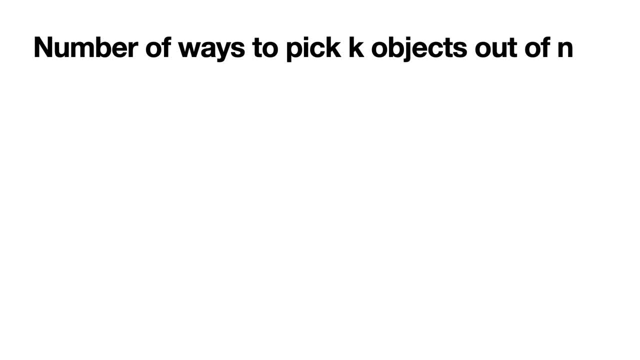 over counting and divided by two removes this over counting. so let me elaborate a little bit more on this way of choosing two elements out of 10.. in the general case, let's say you have a set of n objects and you'd like to be k of them. the number of way of picking this k? 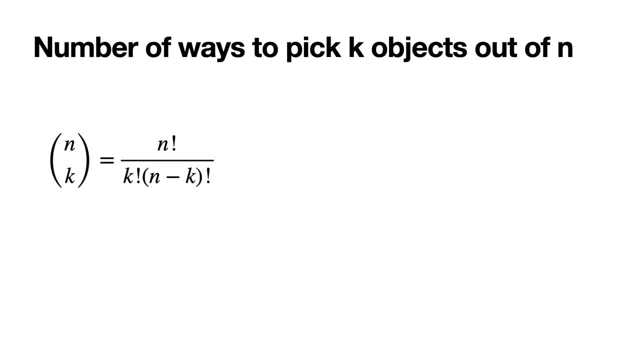 objects is given by the number n. choose k calculated as n factorial divided by k factorial times n minus k factorial for any positive integer. k k factorial is the product of all the positive integers smaller than or equal to k, which is k times k minus 1, times k minus 2, etc. etc. until 3. 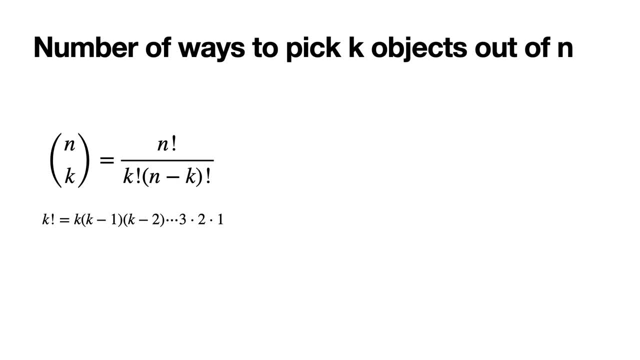 times 2 times 1.. actually, k factorial is the way of ordering k objects in a line. so, for example, what is the number of ways of picking three coins out of a set of 10.. well, that's going to be 10. choose 3, which is 10 factorial divided. 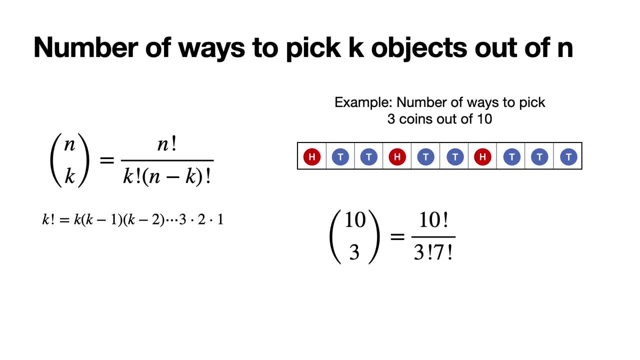 by 3 times factorial, times 7 factorial. if you work out the ratios and cancel a bunch of repeated stuff, you're going to get 10 times 9 times 8, divided by 3 times 2 times 1, and that is one twin and in general, the probability of a coin landing. 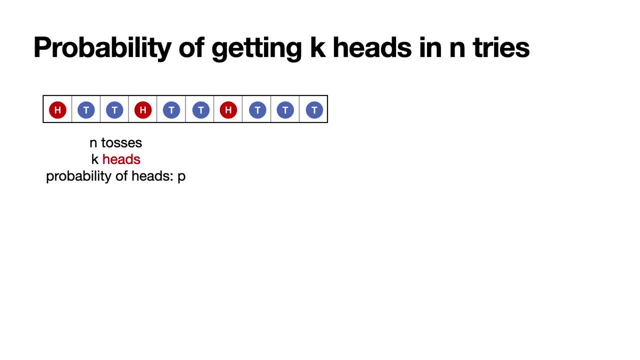 k times in heads in n throws, where the probability of landing in heads once is the number p. is this number over here and choose k times p to the k, times 1 minus p to the n minus k. the first one is the number of ways to pick which k throws are going to be head. the p to the k is the probability. 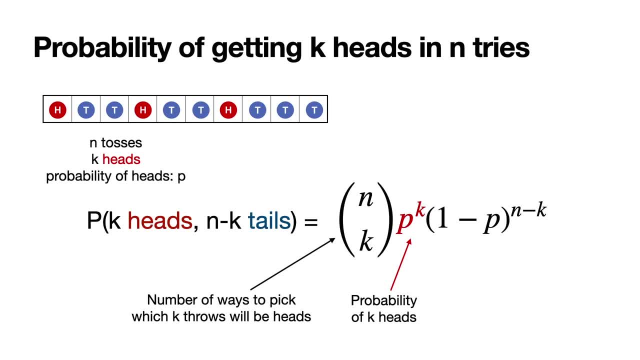 of those k throws that land in head, since each one of them has probability p, and the one minus p to the n minus k is probably the remaining n k throws land in tails, and the probability of one coin landing in tails is 1 minus p, and so this is a binomial distribution with two parameters. 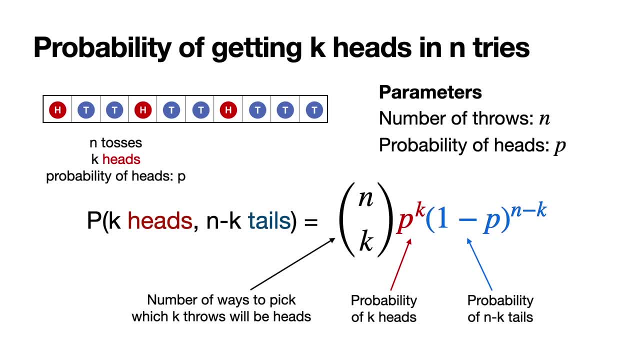 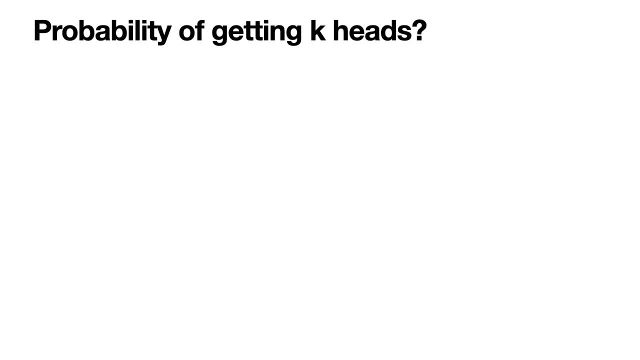 the number of throws, which is n, and the probability of heads, which is p. now, if we calculate these numbers for again, n equals 10 throws and p equals 0.3 probability of landing in heads, and k from 0 to 10, we are going to get 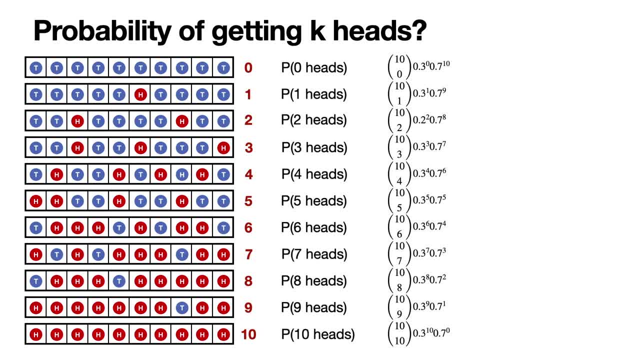 the following numbers: 10- choose 0 times 0.3 to the 0 times 0.7 to the 10 is the probability of 0 heads. 10- choose 1 times 0.3 to the 1 times 0.7 to the 9 is the probability of 1 heads. 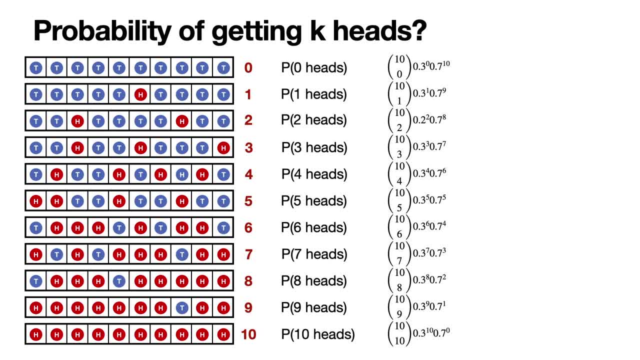 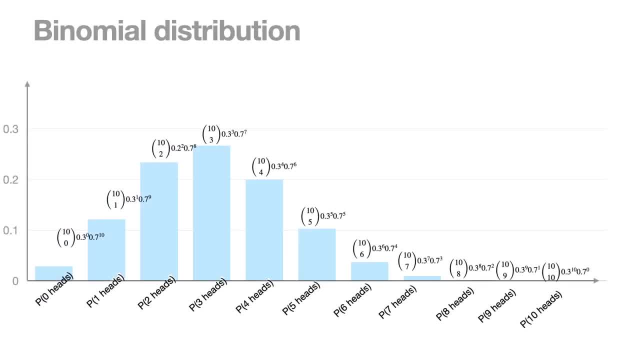 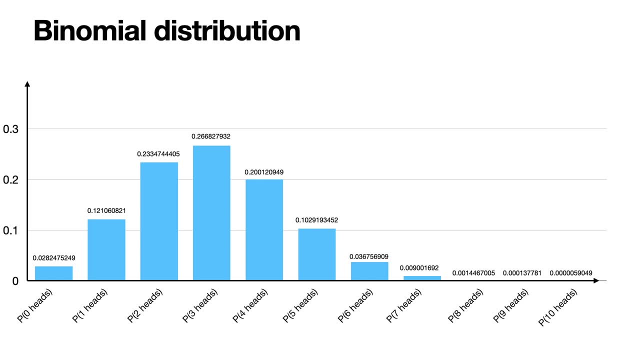 etc, etc, etc. and when we plug these numbers into a calculator, we get these numbers over here that i mentioned before and we put these numbers into a nice histogram. we get these for the probabilities. these are the numerical values, and so that is a binomial distribution. so next i want to do is show you a very, very special distribution called the Poisson. 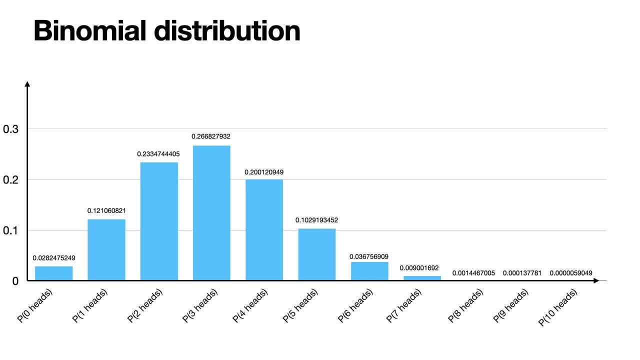 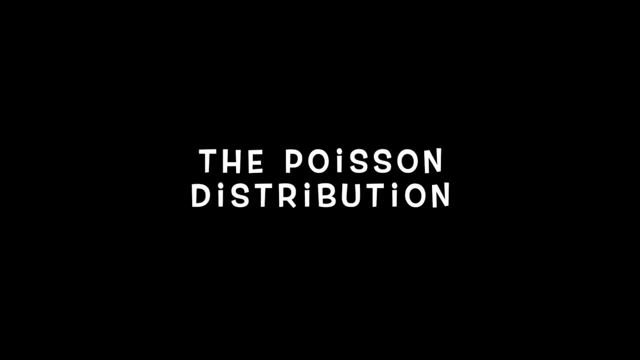 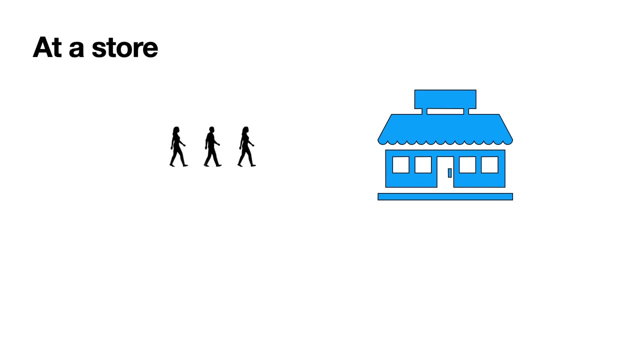 distribution, which can be seen as a limit of binomial distributions, in a very interesting way. so the Poisson distribution answers the following type of question that i mentioned before. imagine that you have a store and throughout the years you see people entering and leaving and you take. 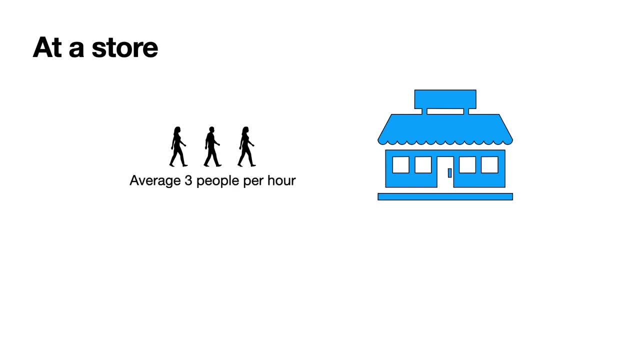 an average and notice that on average, in particular hours, three people enter the stores. And now the question is the following: Given this information, what is the probability that over the next hour, five people will enter the store? So the number of the following. 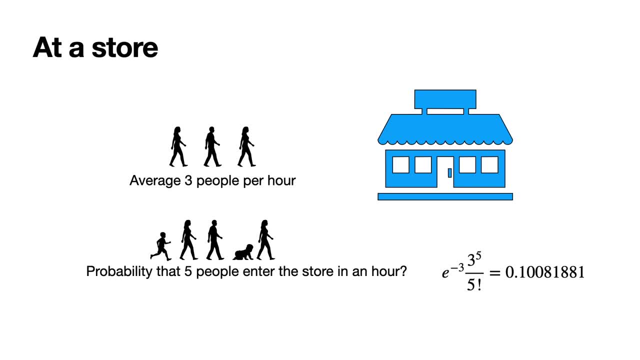 It's e to the negative three times three, to the five over five factorial, which is 0.1008, et cetera. E over here may look familiar. It's the Euler number 2.7182, et cetera. 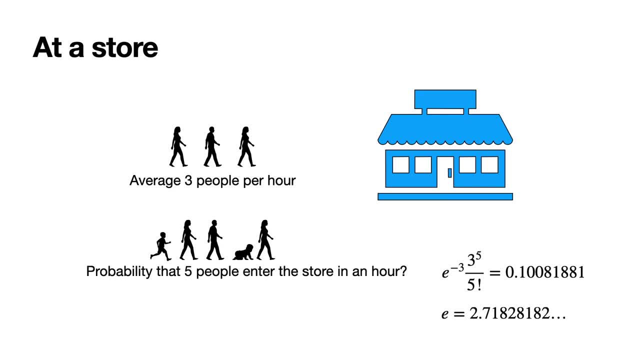 And it's one of the most important numbers in mathematics and statistics and physics and many, many, many fields. I would say it's up there with pi. But the great thing is that this formula is universal. The three and the five are arbitrary. 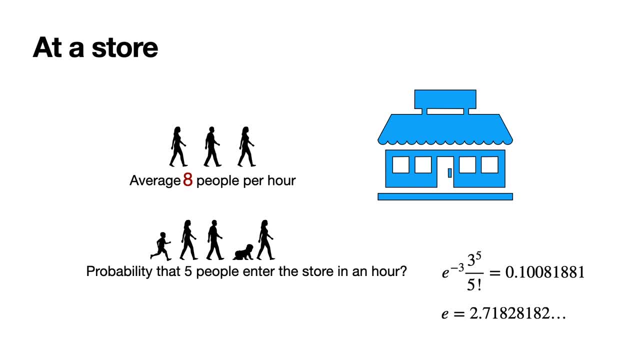 If you counted and said that eight people arrive every hour and what's the probability that two people enter the store over the next hour, That's e to the minus eight times eight squared over two factorial, which is 0.01073, et cetera. 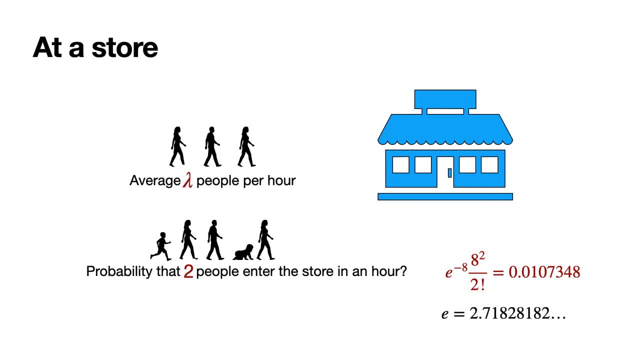 And in general, if the average number of people that enter per hour is lambda and you want to find out the probability that K people enter the store in the next hour, then that number is e to the negative. That's e to the negative. lambda times, lambda to the K over K. factorial. 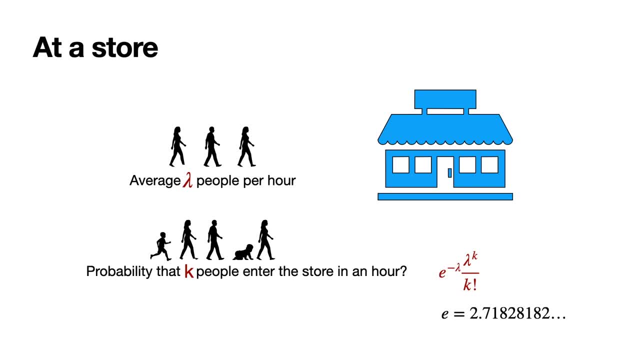 That is precisely the Poisson distribution. Now the question is: how do we calculate this number? The expression was complicated, but actually follows from binomial distribution using a limit. Let me show you how. So, in order to solve this problem, we're going to start with a simple one. 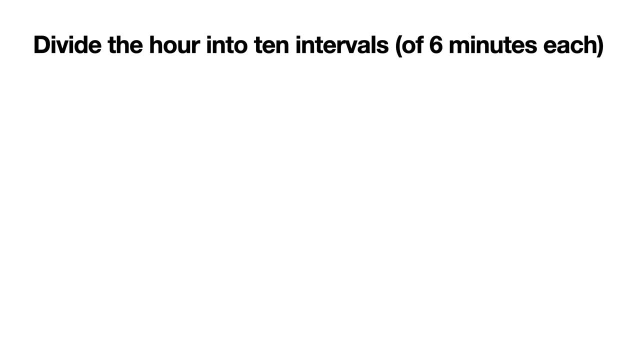 Imagine that in our store we don't really want that many people at the same time. Maybe there's a pandemic and we can only have one person at a time. So we open 10 intervals of six minutes each and only one person can come. 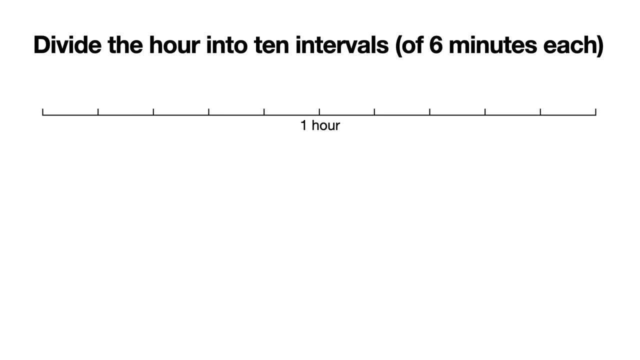 at each interval and they must leave when the interval finishes. Now, in this simplified problem, we keep track of visitors and find out that, on average, three people are visiting the store per hour. Does this problem sound familiar? Well, it's very similar to the one of the coins. 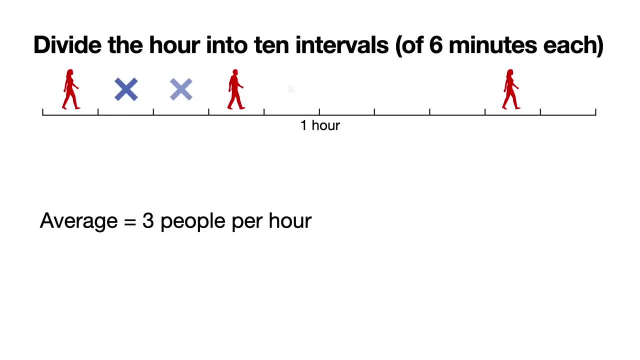 because take a look at all the other intervals. Nobody arrived at any of those seven intervals. That's the same as tossing a coin 10 times and the coin landing in heads- three times, corresponding to each of the times a person entered the store, and in tails, seven times corresponding to each. 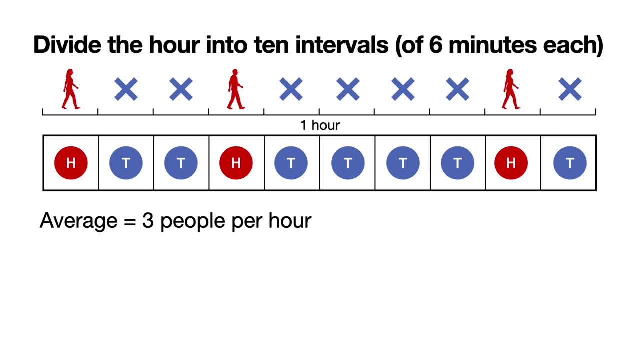 of the times a person did not enter the store. So we know that probability. That's the same as the probability of getting heads three times And that's the binomial distribution, where p of heads is 0.3 and p of tails equals 0.7.. 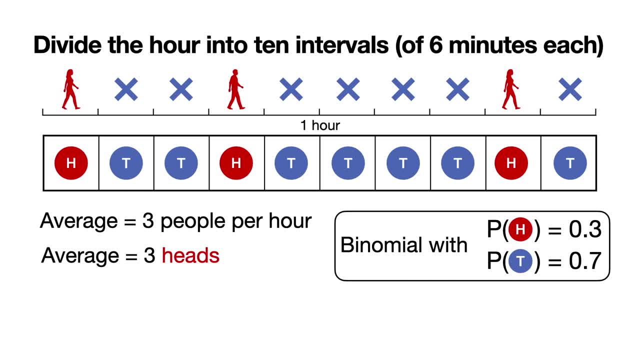 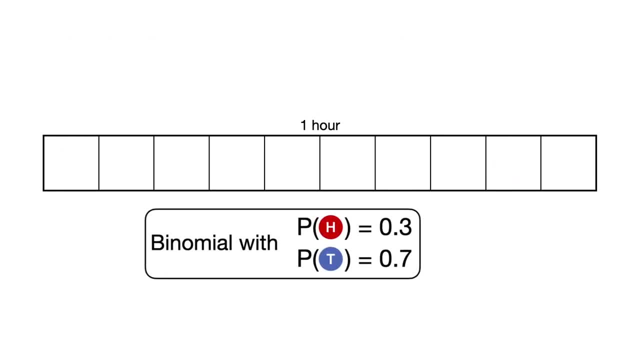 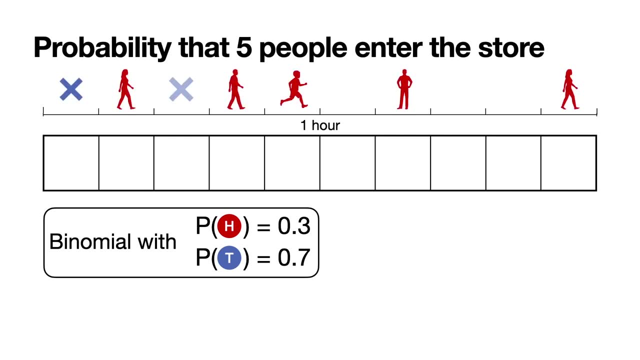 So, in this particular problem with the intervals, the number of people arriving in the store is modeled by the binomial distribution. So, for example, what's the probability that five people enter the store in the next hour? Well, that's the same probability that we toss a coin 10 times and that the coin 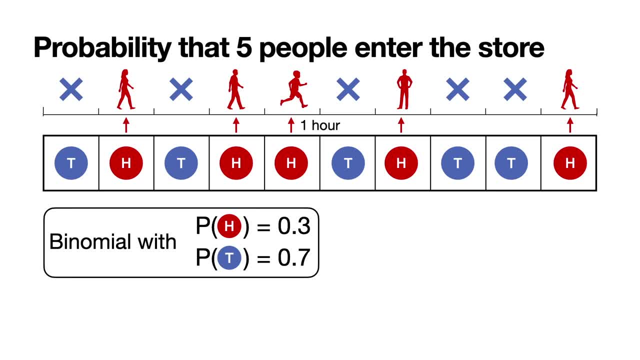 lands in heads five times corresponding to the times that people arrived, and in tails another five times corresponding to the intervals where nobody arrived. And so the probability that five people arrive over the next hour is the same probability that if we throw this coin 10 times. 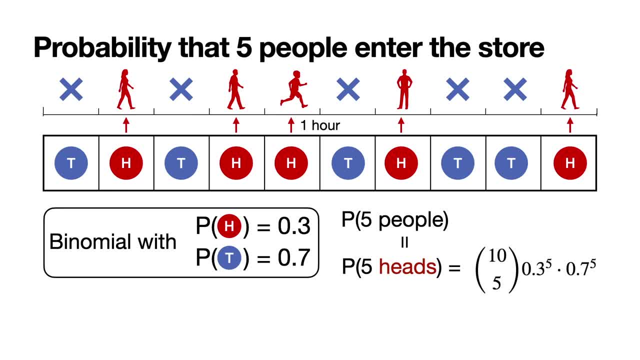 it coin lands in heads five times, And that's 10. choose five times 0.3 to the five, times 0.7 to the five, Where again these 10 choose five: the number of ways to pick the intervals in which five people arrive. 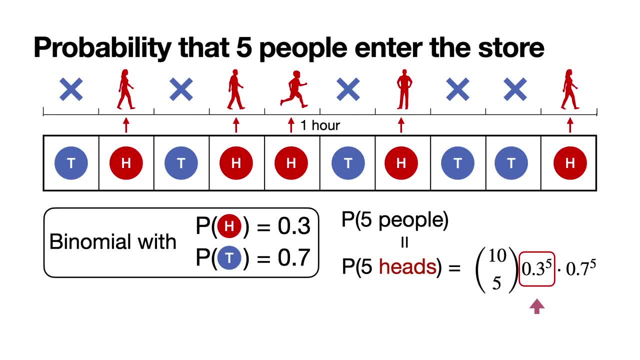 this 0.3 to the five is the probability that people arrive at those intervals, And 0.7 to the five is the probability that nobody arrived at the other intervals. Now, something very important here is that this 0.3 is 3 over 10 and this 0.7. 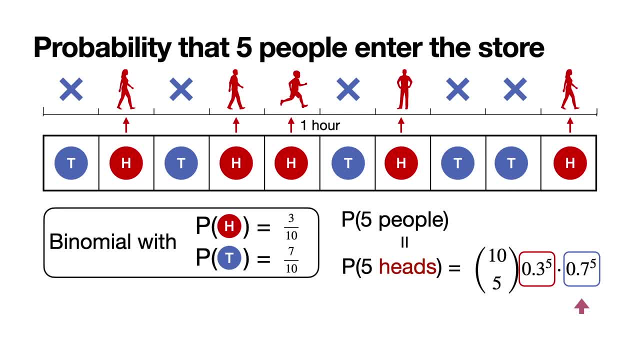 is 7 over 10.. So now we're going to do is we're going to change this 10 to different numbers- 20 and 60 and anything we want- and these probabilities are going to change. So let's say that we realize that 10 intervals is too little. 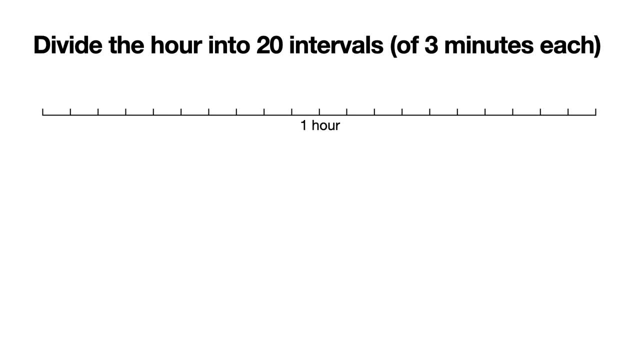 So we decide to divide the hour into more intervals, say 20 intervals each of three minutes. And what happens now? Now we want the probability of five people will enter the store over the next hour. Well, just like before, except that now. 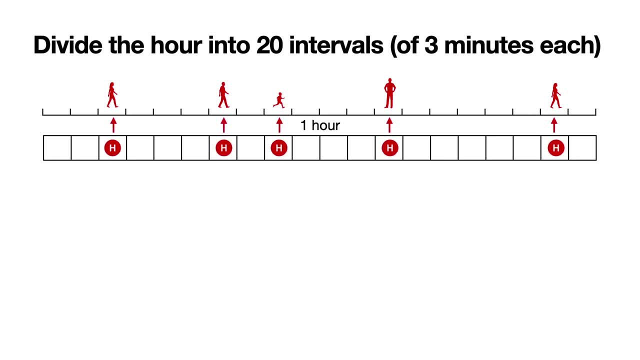 we throw the coin 20 times. it lands on heads five times and on tails 15 times for all the times that nobody entered the store. But now, what's the probability that the coin lands in heads or tails? Well, recall that, on average, 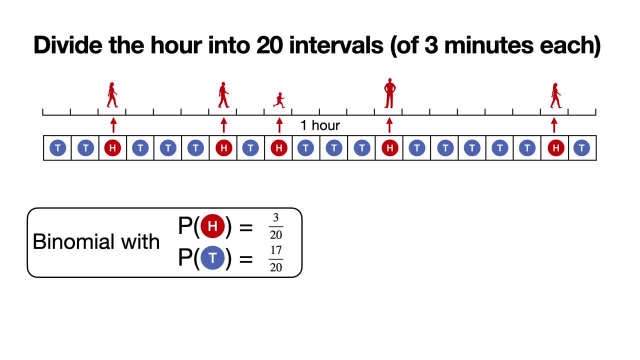 we still have that three people enter the store at every hour. This still happens, And so, therefore, this is a binomial distribution where the probability of heads is now 3 over 20 and the probability of tails is 17 over 20, because, on average, 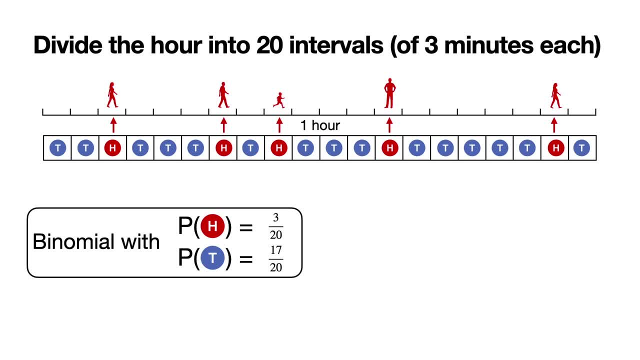 three people enter the store. That means that on average, the coin lands in heads three times out of 20.. And that means that the probability of heads is 3 over 20 and the probability of tails is one minus that, so it's 17 over 20.. 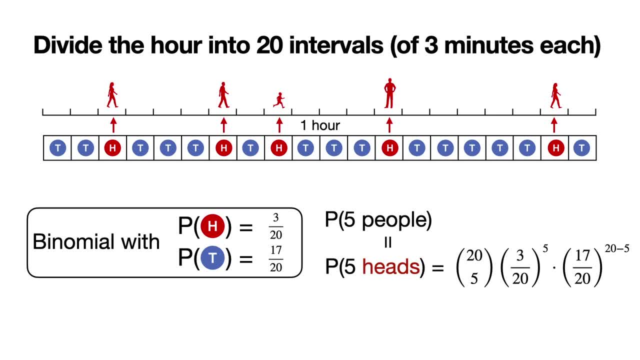 And on this binomial distribution, the probability that five people arrive over the next hour is the same as the probability that five coins landing in heads, which again is 20. choose 5 for the positions, times 3 over 20 for the probability that people arrived and. 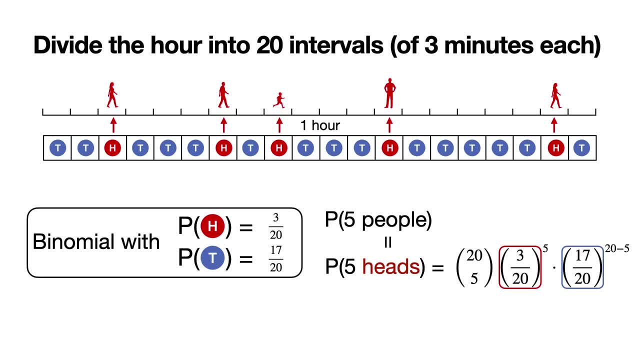 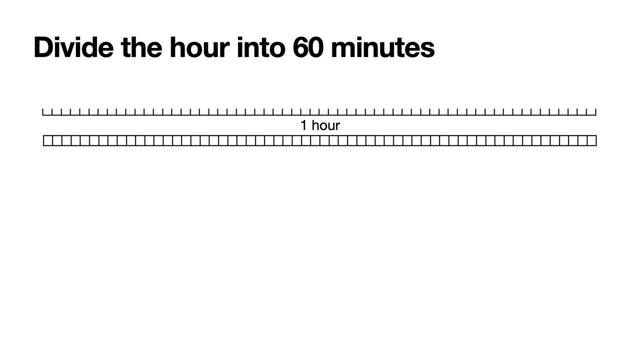 17 over 20 for the probability that people did not arrive, And we can continue doing this. We can subdivide the hour, let's say now, into 60 intervals of one minute each, And so now we have this binomial distribution with probability 3 over 60. 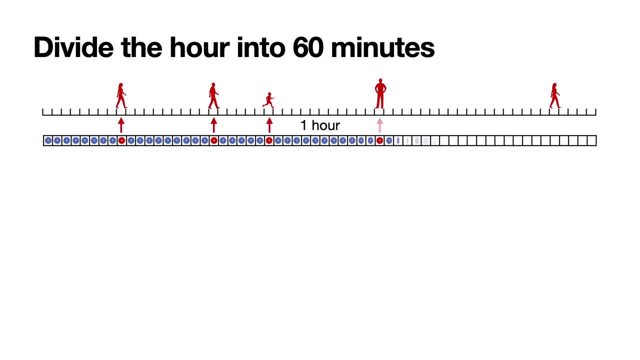 of landing heads and 57 over 60 of landing tails And we want the probability that we toss this coin 60 times and it landed on heads five times, So that's going to be 60. choose 5 times 3 over 60.. 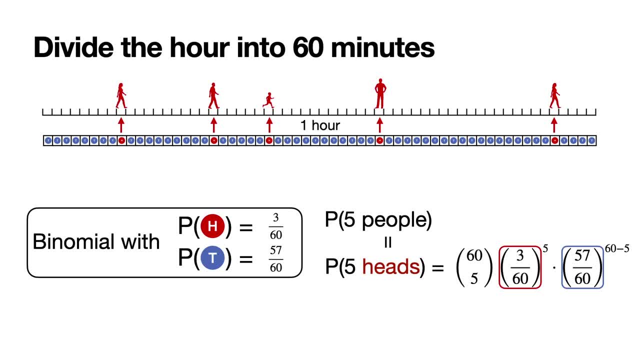 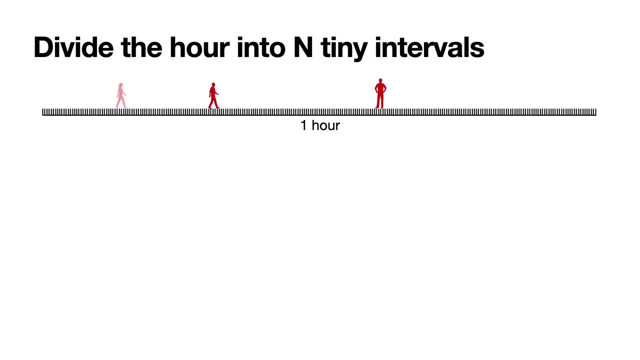 To the five times 57, over 60 to the 60 minus five, And we can continue doing this, and even smaller and smaller and smaller intervals. So let's say there's n of them. I want to see the probability that five people arrive. 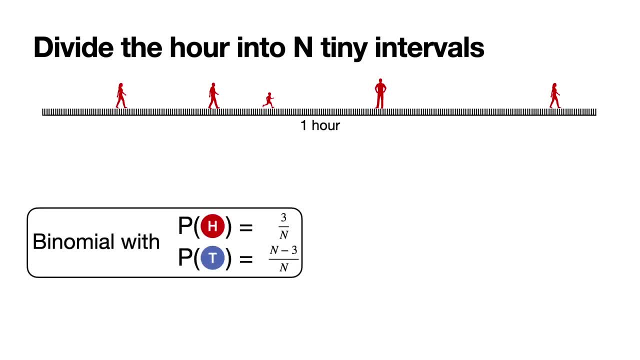 And the binomial distribution is the one where p of heads, or p of person arriving, is 3 over n in an interval, and p of tails, which is no person arriving at that interval, is n minus 3 over n. So the probability that five people 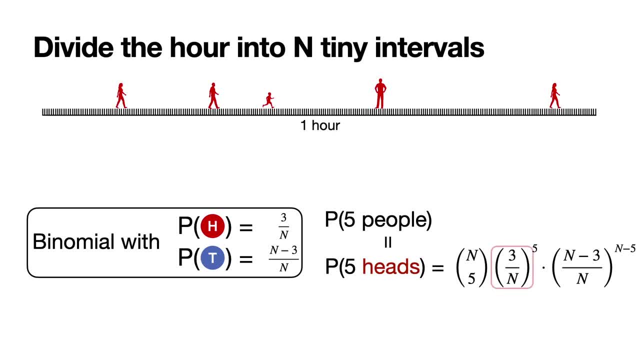 arrive in this binomial distribution is n choose 5 times 3 over n to the 5 times n minus 3 over n to the n minus 5.. And so now, basically, we're going to let n go to infinity, because if you imagine, if n is infinity, then that's the original. 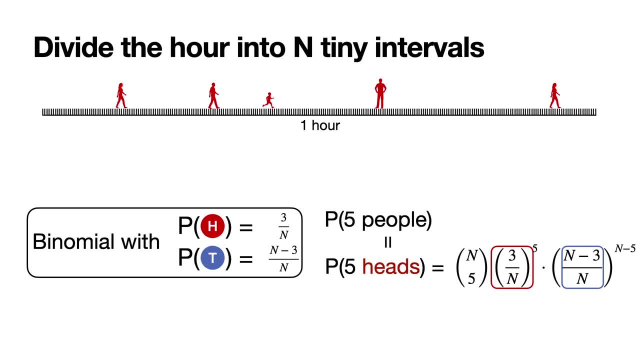 problem, because people can arrive pretty much at any second of the hour or any instant, And so what we need to do is let n go to infinity and see where this formula goes. So first let's look at some numbers, And these numbers are the probabilities we 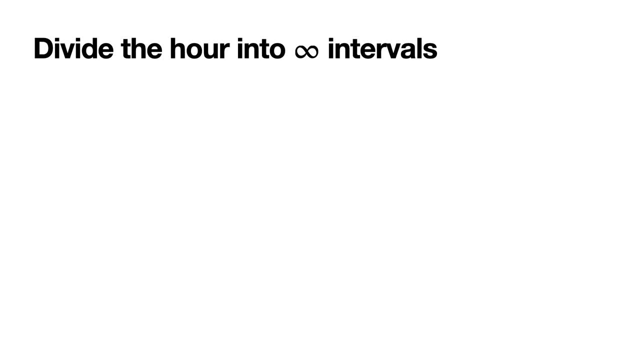 obtain when we split the hour into different numbers or intervals. So when we split the hour into 10 intervals of six minutes, the probability of five people arrive is 10. choose 5 times 3 over 10 to the 5 times 7 over 10 to the 5,. 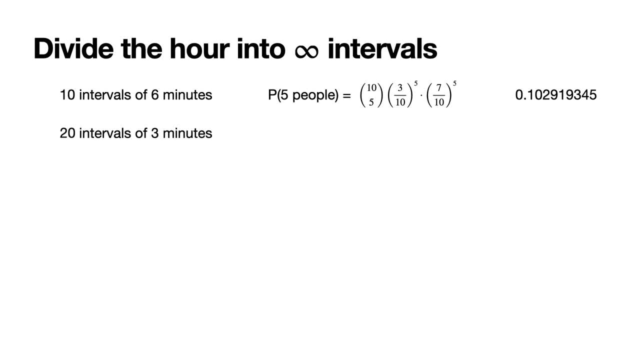 which is 0.1029.. If we divide into 20 intervals of three minutes, then this is the formula which is 0.1028.. If you divide into 60 intervals of one minute, then it's this number which is 0.1028.. 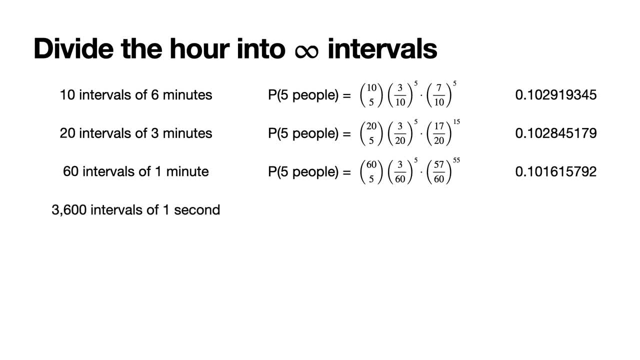 If you divide into 16,, if you divide into 3600 intervals of one second, then this is the number and it's 0.1008.. So these numbers are sort of converging somewhere. Let's say we divide it into 3,600,000 intervals of one millisecond. 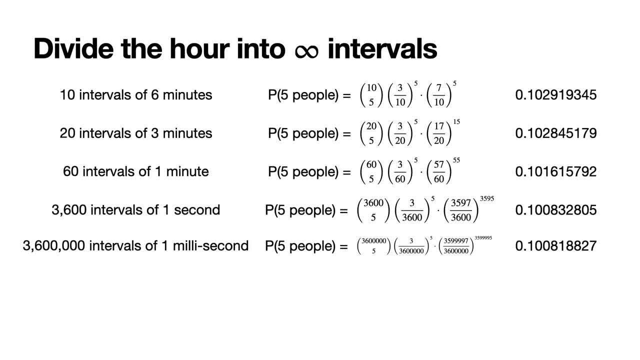 This is the probability now, and that's 0.1008, et cetera, et cetera, And the idea is to see the limit of this. So where do these numbers converge? So, at the end of the universe, at the end of doing this process infinitely, we're. 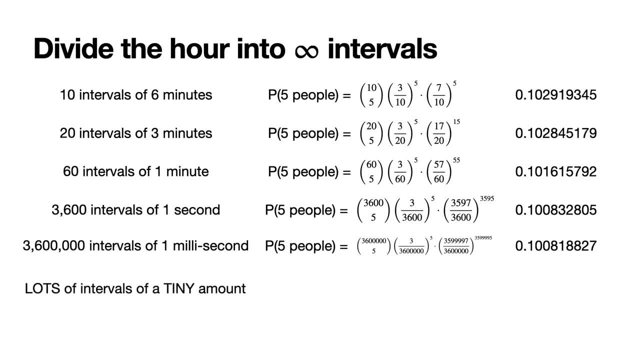 going to have. an interval of one hour splits into lots and lots of tiny, tiny intervals of a tiny amount. In principle, we have infinitely many intervals of length- zero. Now plugging in infinity here is difficult. We're not going to get a number. 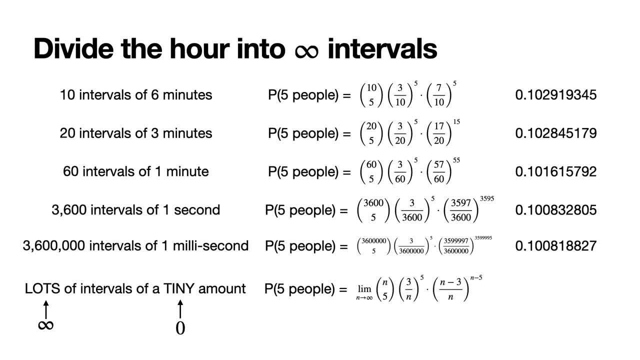 But what we can do is use calculus. We can call it the limit, as n goes to infinity of n. choose 5 times 3 over n to the 5 times n minus 3 over n to the n minus 5.. That is the probability that five people 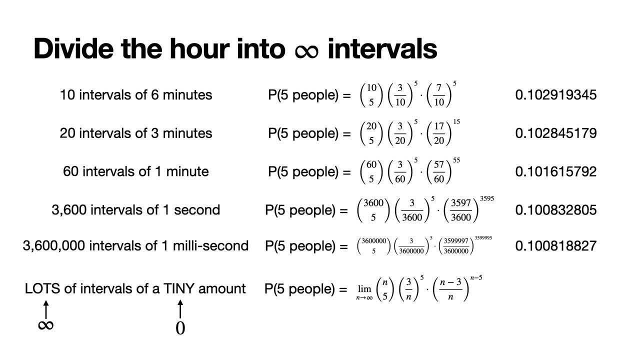 enter the store. if we subdivide it into infinitely many intervals of one instant length- And that's the probability we were looking for at the beginning- This number is 0.1008.. And how do we calculate this number? Well, let me show you some. 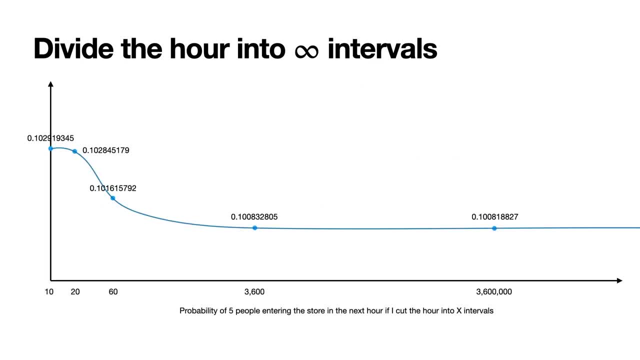 But first let's plot these numbers And notice that the probability of five people entering the store in the next hour is somewhere the limit at the very, very right in this plot. On the horizontal axis we have the number of intervals. On the vertical axis we have the probability. 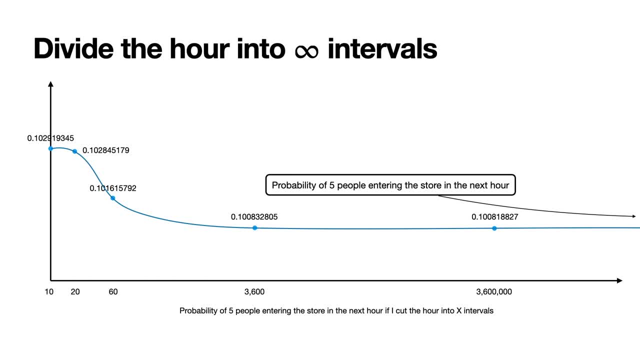 And, as you can see, the horizontal axis is logarithmic, And so the limit is some number over here, where this number is, where this sort of blue line converges in infinity, And the value is 0.1008.. And that is precisely the probability. 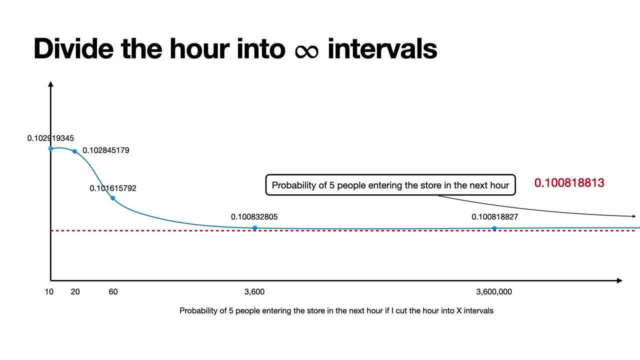 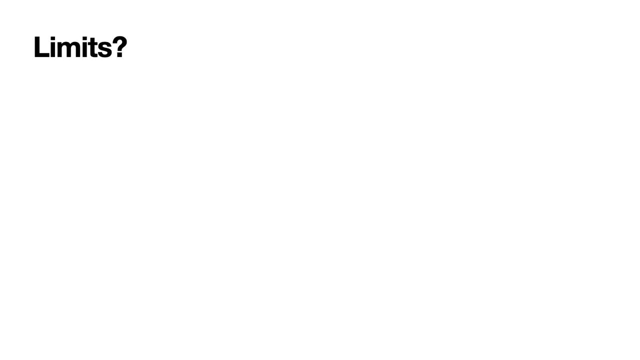 of five people entering the store in the next hour. But now I still haven't told you how to calculate the 0.1008.. So let me show you How, Using algebra. So the way we're going to do it is the following: 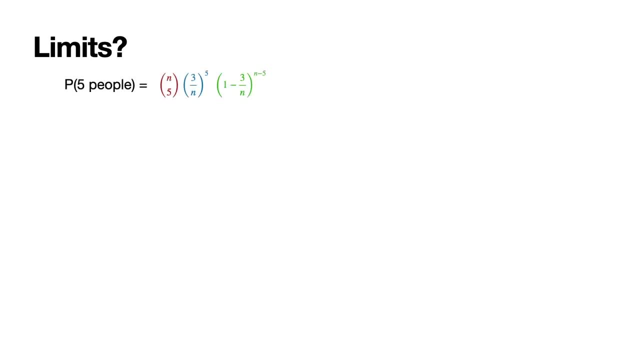 The probability that five people enter the store is n choose five times three over n to the five times one minus three over n to the n minus five. And what I want to show you is that, as n goes to infinity, this actually converges to the expression three to the five over five. factorial times, e to the negative. 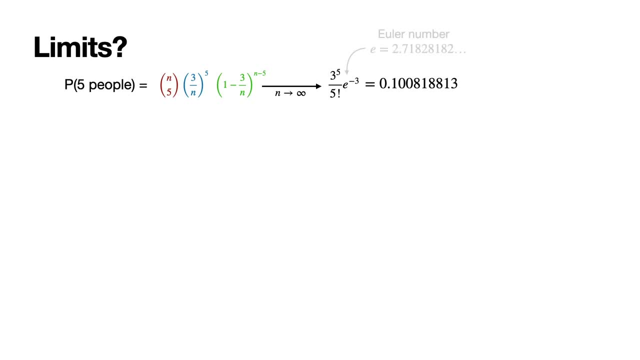 three, which is this number we saw before. Recall that e is the Euler number, 2.71828182, et cetera, which, if you want to know more about it, check out this video that I have over here in my channel where different expressions of e are explained. 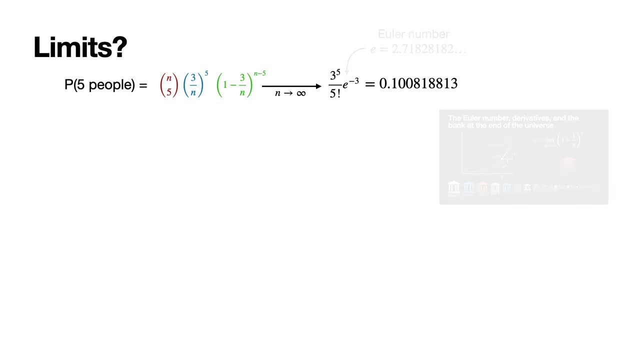 in particular one that we're going to need pretty soon. So let's get back to the math. The red part n choose five can be expressed as n times n minus one times n minus two, times n minus three times n minus four, divided by five factorial. 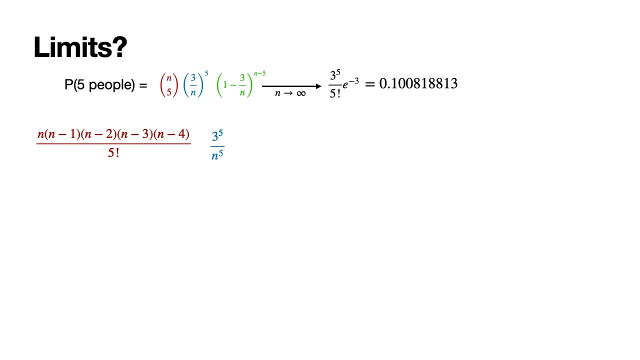 The blue part is three over n to the five, which is three to the five over n to the five, And the green part is one minus three over n to the n minus five. I'm going to take that n minus five and split it into n and minus five. 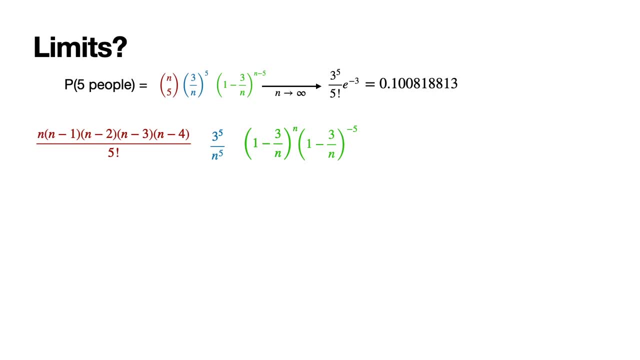 So we get one minus three over n to the n times, one minus three over n to the minus five. Now let's break it down even more. Look at that one minus three over n to the minus five. That one minus three over n can be expressed as n minus three over n. 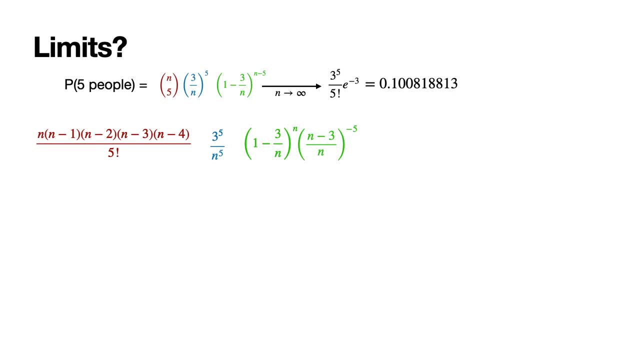 And now let's get rid of that pesky minus five exponent, because that's the same as n over n, minus three to the five. Now we have an n to the five on the bottom and then n to the five on the top, So they get canceled. 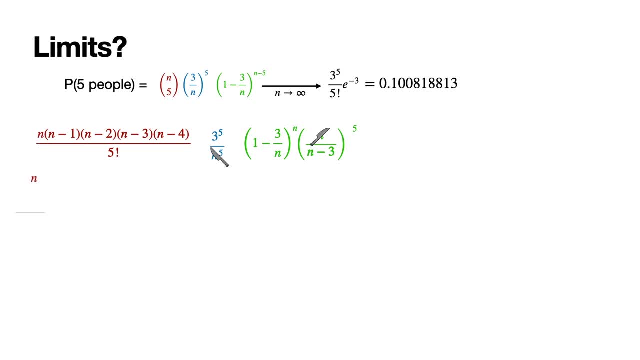 And now let's look again at the red number. These are n times n minus one, n minus two, n minus three, n minus four. We're going to divide them by these five n minus threes. we have over here Now the blue three to the five stays the same. 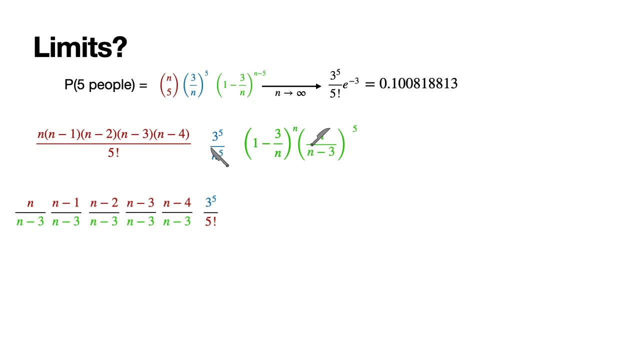 The red five factorial stays the same. And now what remains here is this: one minus three over n to the n. We're going to deal with that in one minute. Now, as n goes to infinity, take a look at any of these numbers. 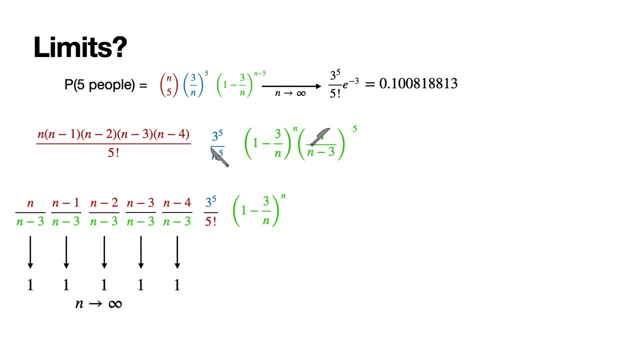 Any of these ratios tend to one because n over n minus three and n minus three get more similar, more similar as they go to infinity in terms of ratio. So all these ratios go to one. when n is humongous, Think about the number ten million. 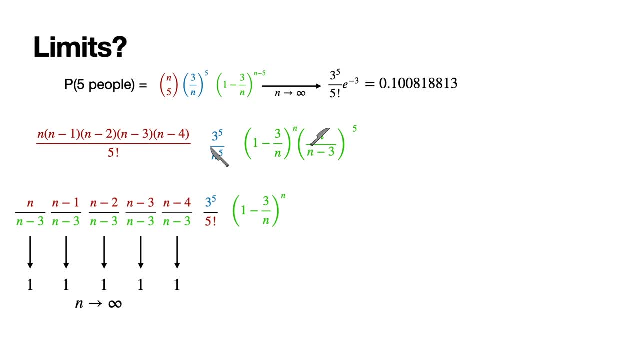 Ten million over ten million minus three is very, very, very close to one, And as n goes to infinity, these are all converging to one. The three to the five over five, factorial stays the same. And now here's the interesting thing. 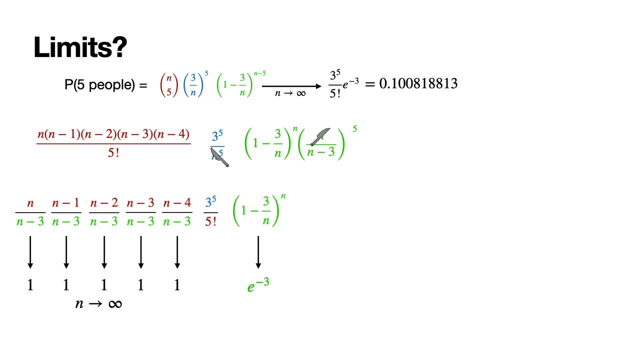 One minus three over n to the n converges to e to the minus three, the Euler number. And again, if you want to see this, check out this video. in there I explain why the limit of one plus x to the n to the n is equal to e to the x. 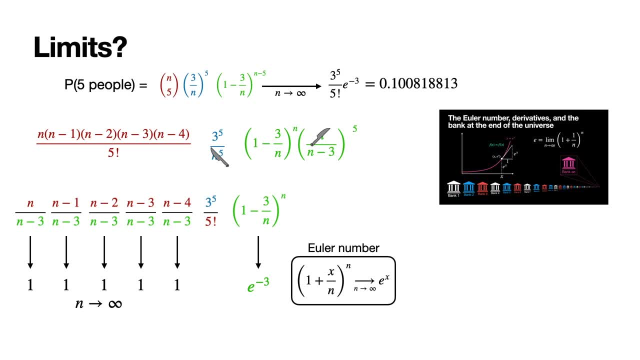 That's one of the main properties of the Euler number. As a matter of fact, it can be one of the defining properties of the Euler number. So that means that this entire product converges to three, to the five over five factorial times e to the negative three. 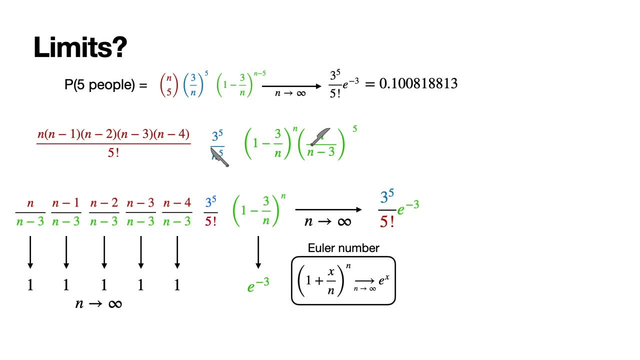 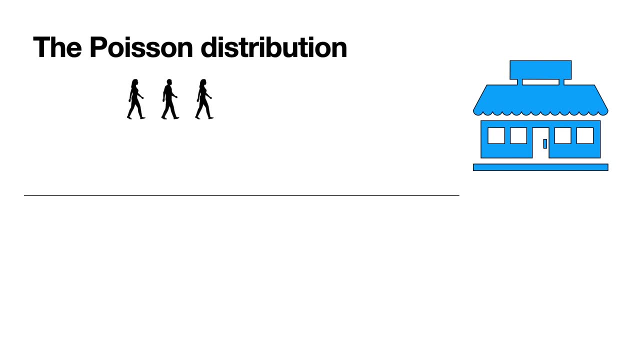 And that number is precisely the number of the probability that five people enter the store in the next hour. So let's recap: You have a store where, on average, three people enter per hour And what's the probability that five people enter the next store in the next hour? 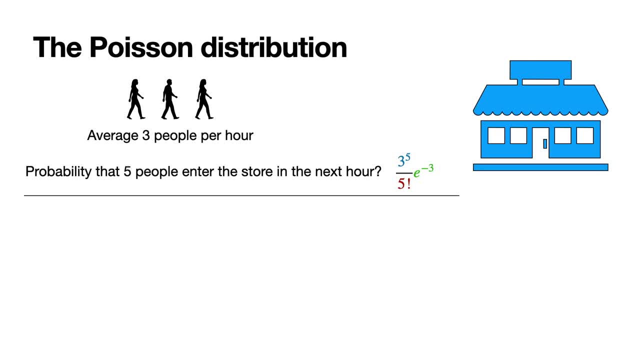 Well, it's three to the five, over five factorial times, e to the minus three. We got that using a limit of over smaller and smaller and smaller intervals. Now what happens if some number lambda people enter per hour where lambda doesn't have to be an? 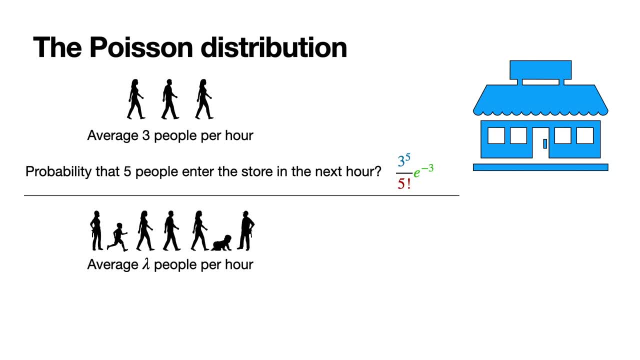 integer, because it's an average, can be seven point three, one, four or whatever. What is the probability then that for some integer k- this time k is an integer that k people enter the store in the next hour? Well, this probability is lambda. to the k over k. factorial times e to the negative. 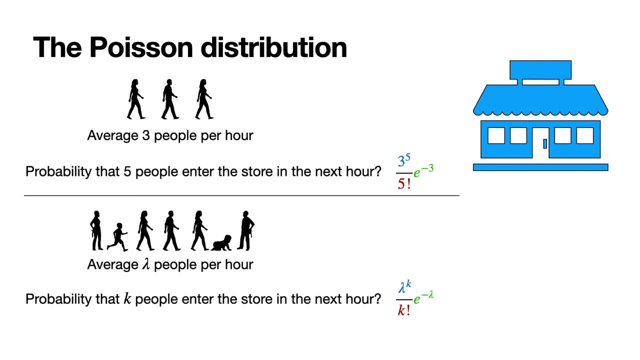 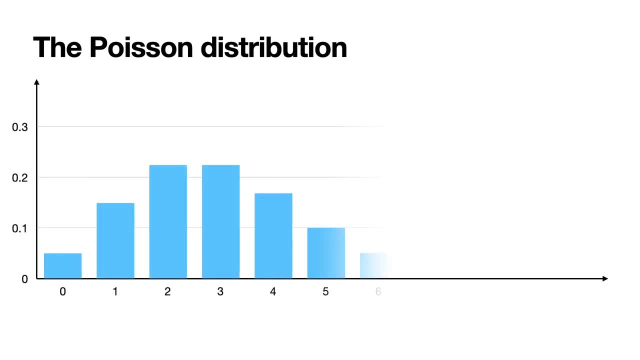 lambda, and all we have to do is the same exact procedure, except change the three to a lambda and the five to a k. And that, my friends, is the Poisson distribution. Here is a histogram of it, where in the vertical axis you have: 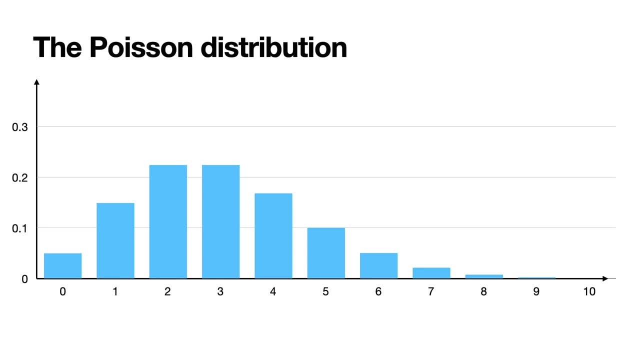 probability, and in the horizontal axis you have the number of people entering the store in the next hour. So here's the probability that zero people enter the store. one person enters the store, two people enter the store, three, four, five, six et cetera, all the way to infinity. 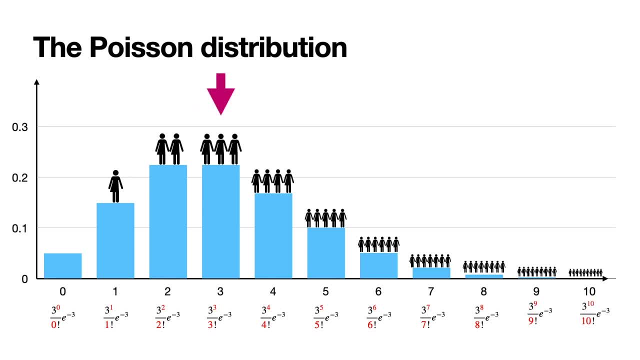 Notice one thing: Notice that the highest probability is at three, because if three people enter the store in an hour, then Most likely three people will enter the store over the next hour. Here, two and three are actually the same, but that's an anomaly. 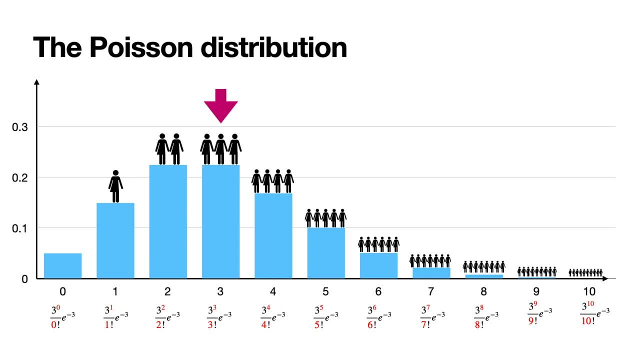 Normally it's the same. is the number of people entering the store The highest probability? Also, notice that all these numbers are actually bigger than zero. So for any n, there's a non-zero probability that people enter the store Now, for example, the probability of five hundred people enter the store in the next. 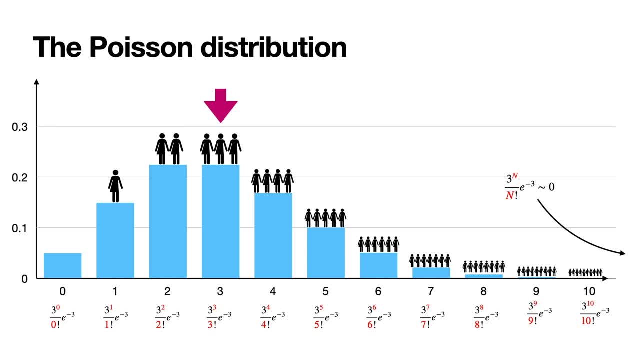 hour is very, very, very tiny, given that only three enter on average, But it's still possible And the probability is just a very, very small number that is bigger than zero. Now notice that all these blue bars add to one, because over the next hour some number of people are going to enter.